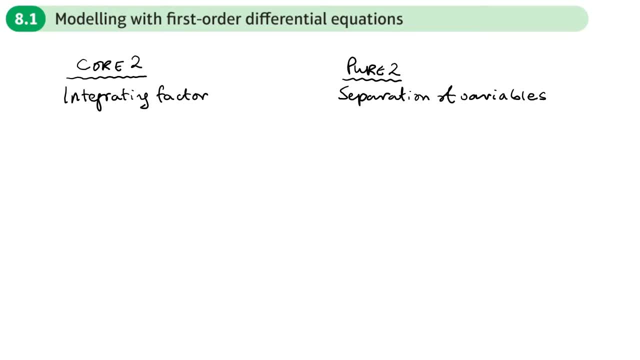 the integrating factor. So just a reminder of the integrating factor, it's when we have a first order differential equation written in this form. so dy, dx plus some sort of function of x, y equals a function, a different function of x and the integrating factor. let's just 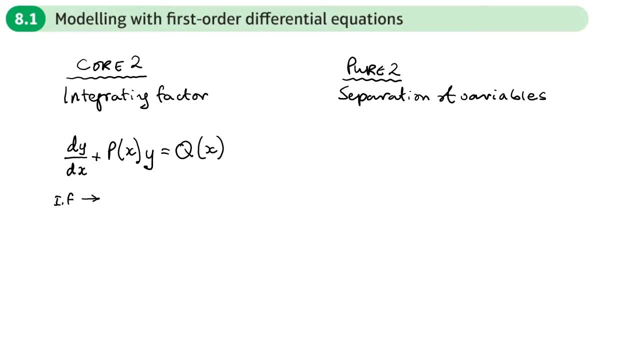 call it the if You get this by doing e to the power of the integral of px dx. Now, just be aware that with a modelling question, we often have things with respect to time. So let's say, for example, that it was volume that we had. 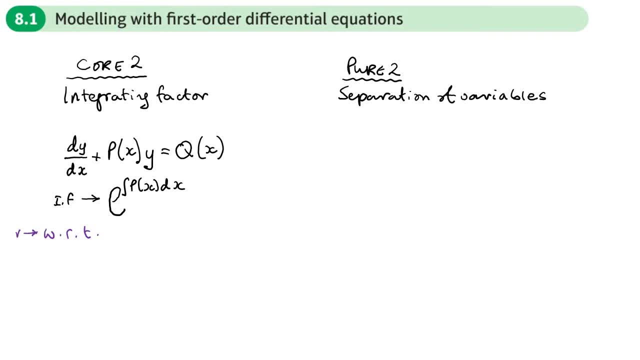 With respect to time. So our differential equation might look something like this: If it was volume with respect to time, then you may see something like this, where v might be volume. yeah, So just be aware that you've got different letters and you need to be prepared. 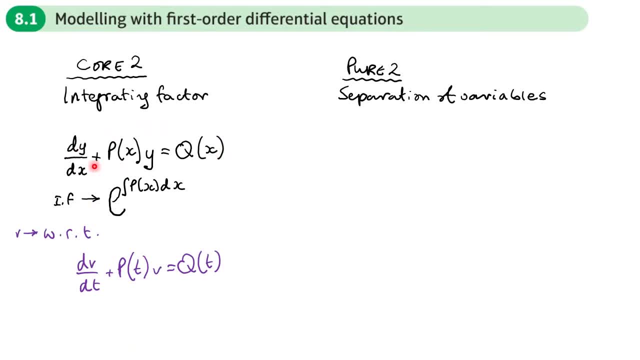 to sort of take what where you're going with respect to time. So what we're going to do here is we're going to take what we're used to and match up the letters for x and y with these, So x, x, x, t, t, t, y, y, v, v. Okay, so that's the only. 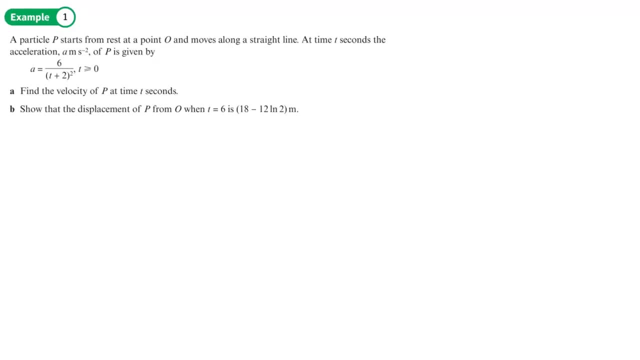 thing you need to watch out for. Okay, so here a particle starts from rest at point zero, which is the origin. So if it starts from rest, It means t is zero. The origin is s equals zero. And this all happens when t is zero, because that's when it starts and it moves on a straight. 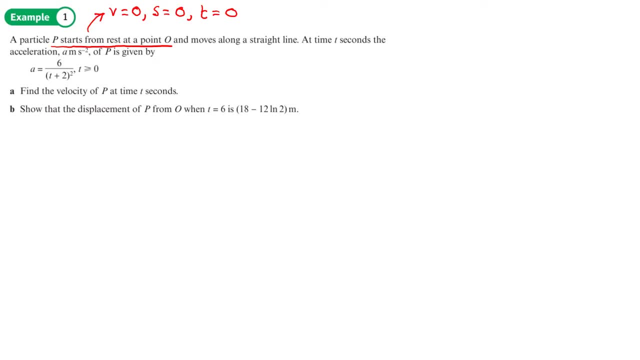 line At time, t seconds. the acceleration is given by this expression here. So we've got the acceleration, find the velocity. So, just as a reminder, when we differentiate the displacement with respect to time, Okay, We get the velocity. When we differentiate the velocity with respect to time, we get the acceleration. 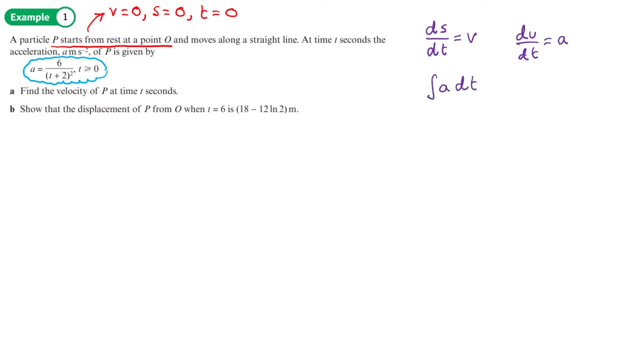 When we integrate the acceleration with respect to time, we get the velocity plus c, Let's call that c1.. And when we integrate the velocity with respect to time, we get the displacement plus a different constant. We'll call that c2.. 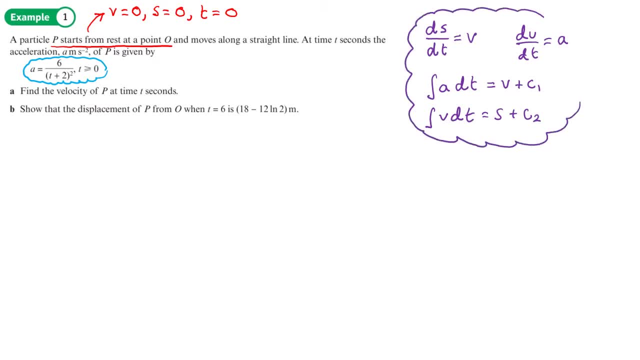 So that's just a reminder Of variable acceleration, which is what we've got. So let's start part a. So if we want to find a velocity at of p at t seconds, then the velocity is equal to what we get when we integrate the acceleration with respect to time. 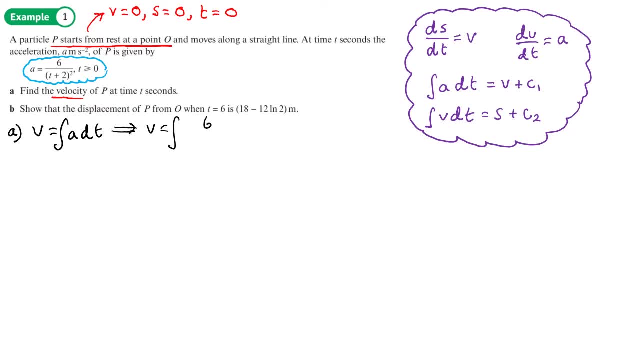 So that's going to be equal to integrating 6 over t plus 2.. Okay, So that's going to be equal to t plus 2 squared dt. So let's write the power as t plus 2 to the negative 2 dt. 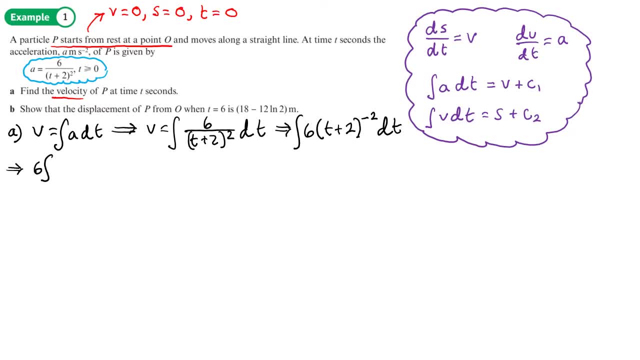 We'll move the constant over just to make it slightly easier. Okay, So that's going to be equal to t plus 2 to the negative 2 dt. So that's going to be equal to t plus 2 to the negative 2 dt. 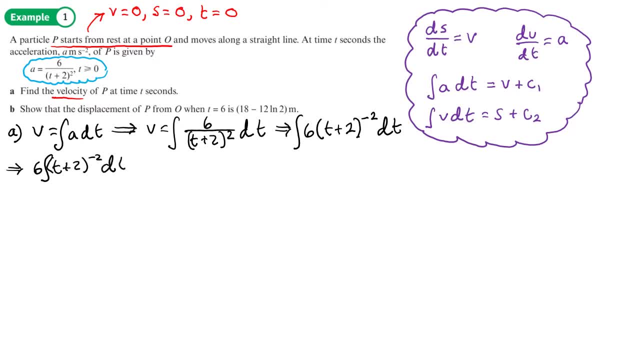 Okay, So we get this, And then we can use the reverse chain rule to integrate what's here. So we add 1 to the power divided by the new power, So we integrate the outside. So that would give us negative t plus 2 to the power, negative 1.. 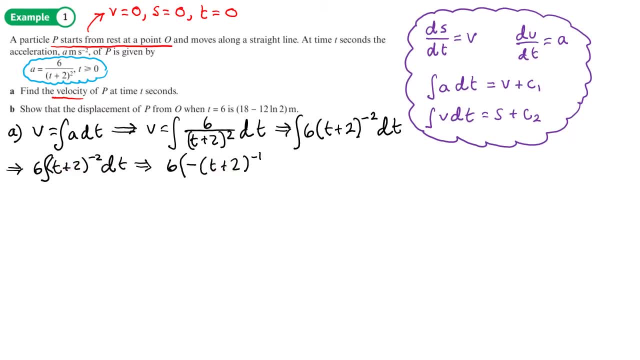 Then we times by the inside integrate differentiate, which is just 1.. So we just get this Plus 1.. plus C, which is what V is. so let's tidy that up. so we've got negative 6 T. actually let's write it as V equals negative 6 over T, plus 2 plus C. so now, 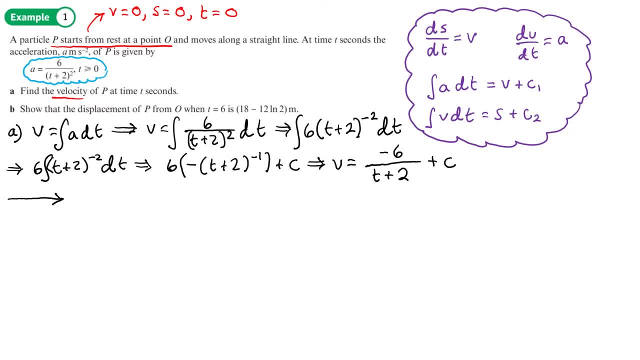 we're going to work out C and we can work out C using the information that's here. so we know that when T is 0, V is 0, so let's write that down: T is 0, V equals 0, so we'll substitute those in to find C. so I'll give a 0 equals negative. 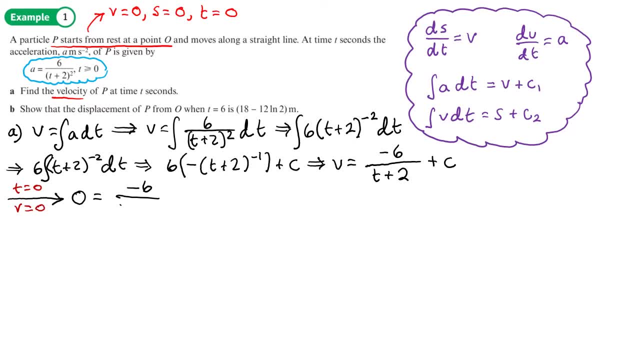 6 over 0 plus 2 plus C. so that just gives us there that C equals, that's going to be 3, C equals 3. so our final expression for V is going to be negative: 6 over T plus 2 plus 3. 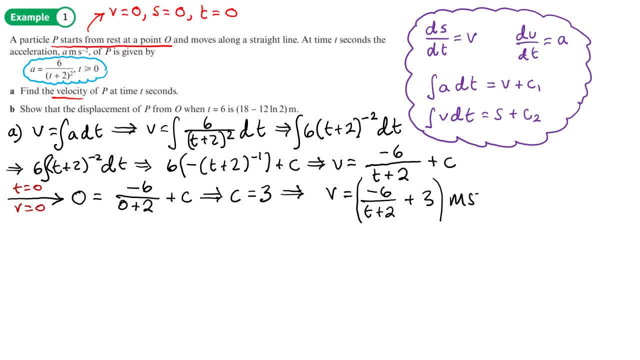 and that is meters per second as its a velocity. so let's just highlight that before we move on. okay, and what I'm going to do, I'm going to call these constants here C 1, as I'm going to be using another constant in part B and I don't want there to be any. 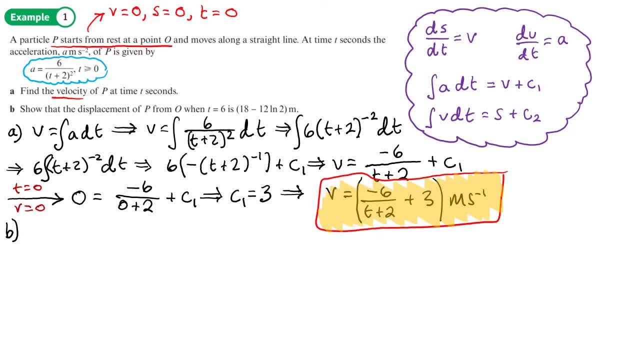 confusion. so part B per second Show that the displacement of P from O when T is 6 is given by that. So if we want to find a displacement, we want to find S. It means we integrate the velocity and we're going to get a constant there. 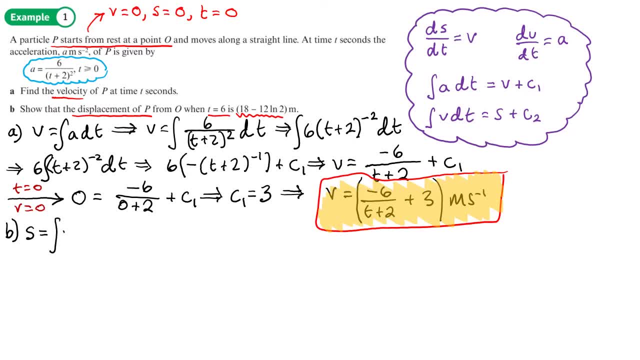 So the displacement S is given by integrating the velocity with respect to time. So S is going to equal integrating negative 6 over T plus 2 plus 3 with respect to T. And we'll do that down here Now for this part, here, when we integrate it, 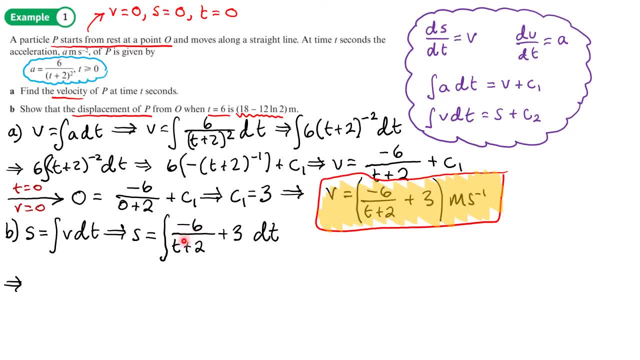 we're going to integrate it with respect to T. So S is going to be equal, integrating negative 6 over T plus 2 plus 3 with respect to T. I'm going to do log of the bottom. So if I did log of the bottom, that would give me 1 over T plus 2.. 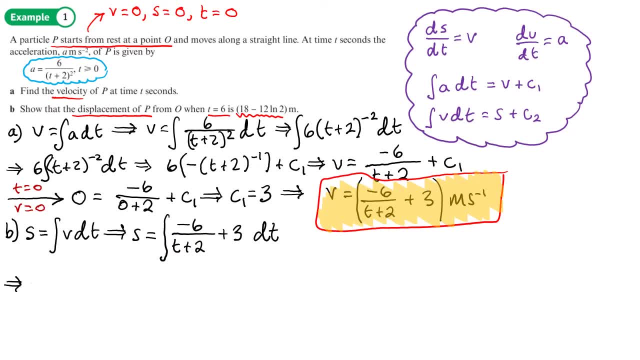 So I've got to times it by negative 6.. So the first term integrated becomes negative 6, log T plus 2. And the 3 will just become 3T plus C. OK, so this is what S equals. I've been given some initial information. back at the top again. 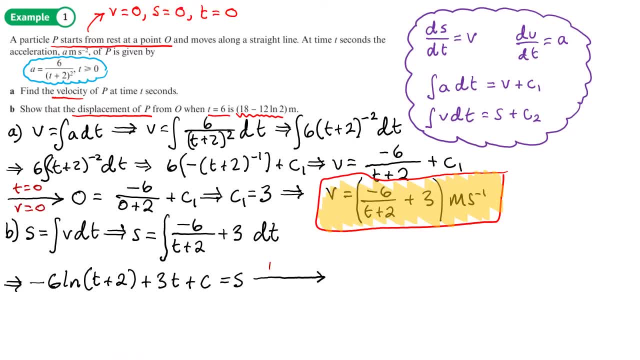 When S is 0, T is 0. And I'll substitute that in so that I can find C. So that will give me: Let's start with S. So 0 equals negative 6 log. I've got to add log 0 plus 2 plus 3 times 0 plus C. 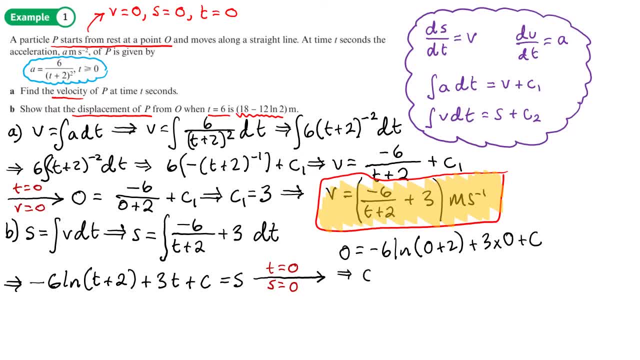 So from that, let's see what do we get? 4C that will cancel out. This will give me negative 6 log 2.. So if I bring it over to the other side it will be 6 log. 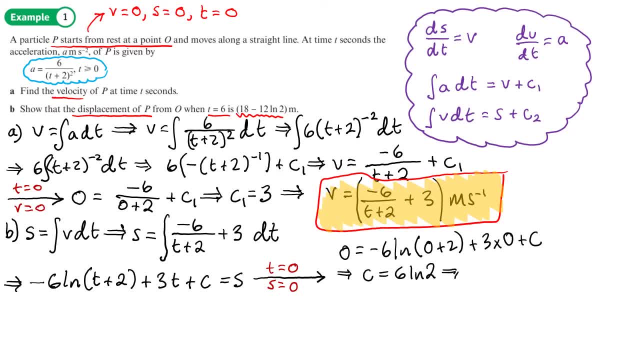 2.. So my full expression for S is negative 6 log. I'm not sure why I'm putting brackets in Negative 6 log T plus 2 plus 3T plus 6 log 2.. OK, now there's. 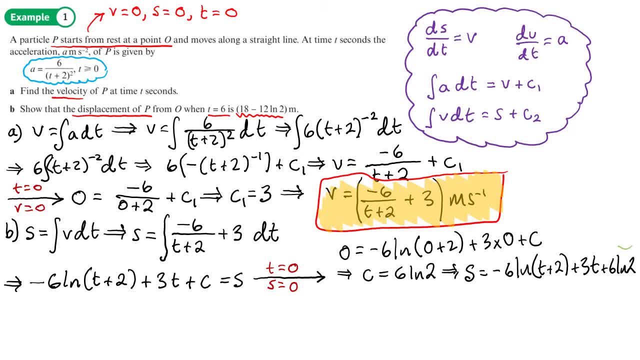 No point trying to simplify that, because I'm now going to substitute in T equals 6.. So let's put T equals 6 here, So S equals negative 6 log 6 plus 2.. OK, Plus 3 times 6 plus 6 log 2.. 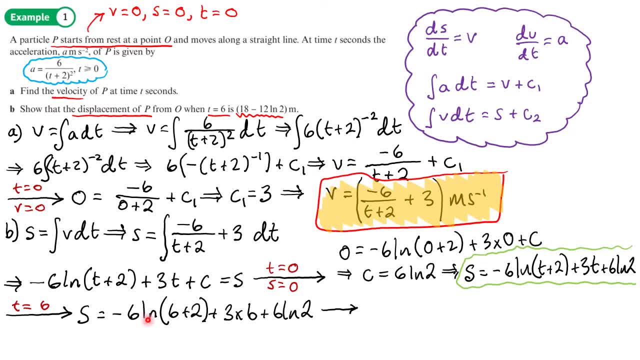 So from there this will just become negative: 6 log 8 plus 18 plus 6 log 2.. Now 8 is the same as 2 cubed, So what I can do is write this as log 2 and times by 3 here. 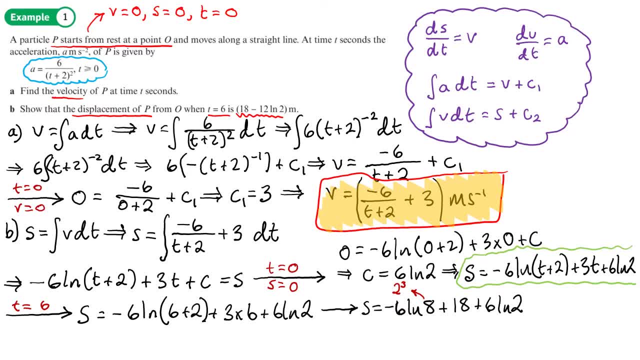 So I get negative 18, log 2.. It's the same thing. So I have S equals negative 18, log 2 plus 6.. log 2 plus 18. then that will give me the form required, because now I can put these together because they're both log 2. so I'll end up with s equals 18 plus. 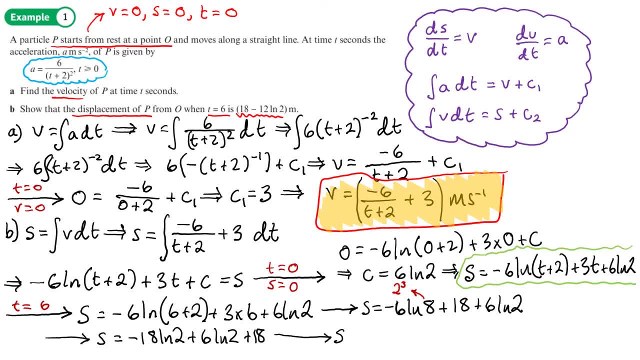 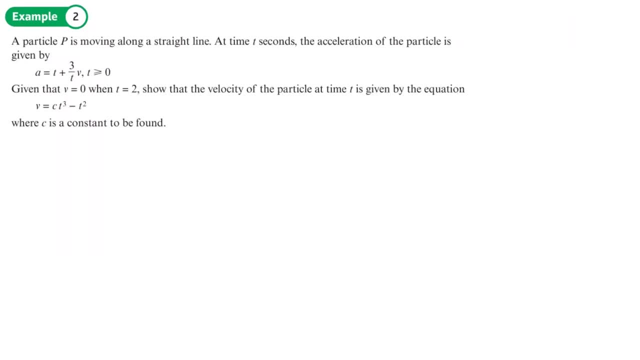 or minus 12 log 2, so s equals 18 minus 12 log 2, as required. okay, so we've got particles moving along a straight line at time t seconds. the acceleration is given by this expression here, given that when the v is 0, when t is 2, show that the velocity of the particle at time t is given by this equation. 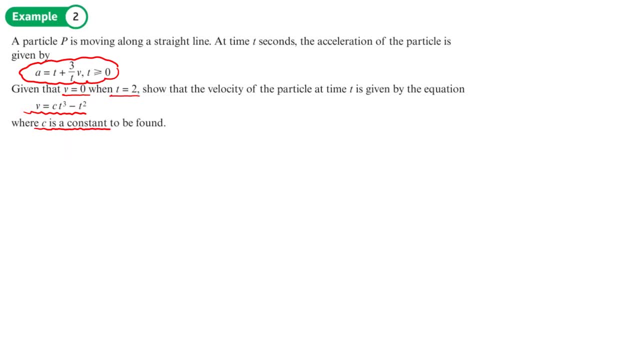 where we need to find the value of this constant c. now, if we look at this, we know that if we want to find the velocity, that's what we get when we integrate the acceleration with respect to time. way of saying that is that dv dt equals a. Now the way this equation looks at the 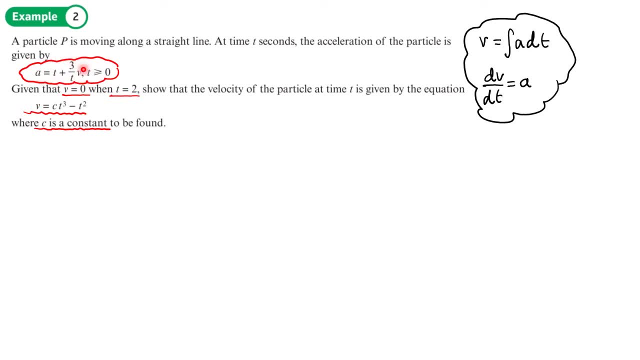 moment or its formula looks at the moment. we can't solve it because we've got t as a variable, we've got v as a variable and we've got a as a variable. we need to eliminate at least one of those. then we can eliminate the a well. 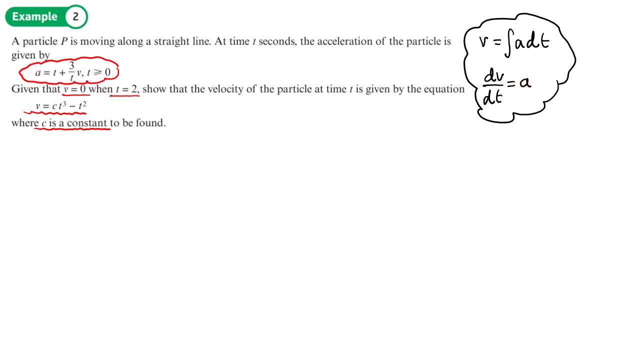 not really eliminate it, but change a to dv dt. yeah, because we can't deal with something with three different variables. so a I'm going to write as. so if I write since a equals dv dt, then I can write dv dt equals t plus 3 over t. 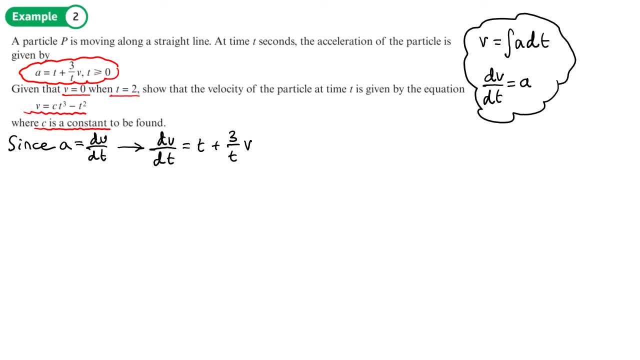 equals t plus 3 over t v. okay, that's that number one. now you might look at this and you might think: okay, let's try a separation of variables to solve this. well, you can't do it because you're not going to be able to get the T isolated from the V. yeah it. 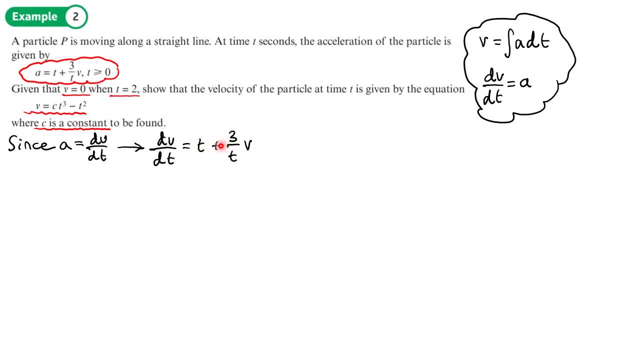 doesn't matter how you try factorizing, it's not going to work. and because this is core 2, this is going to be another method other than what we would use in pure 2 separation of variables. so the method we know is about the integrating factor. now, if we were to write down what the when we use the integrating factor, 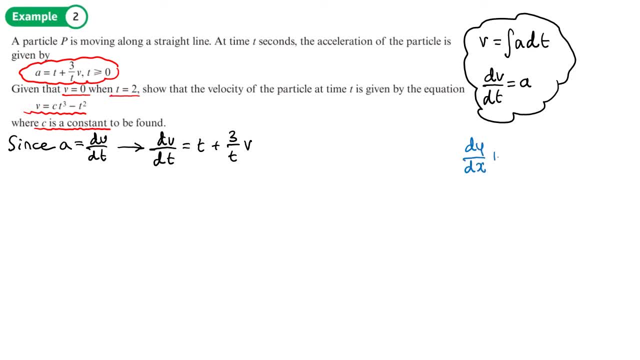 so that's when we've got dy. dx plus a function of x times by y equals a different function of x. you'll notice that this looks a bit like this: now we haven't got X's and Y's, we've got V's and T's. so let's write this using V and. 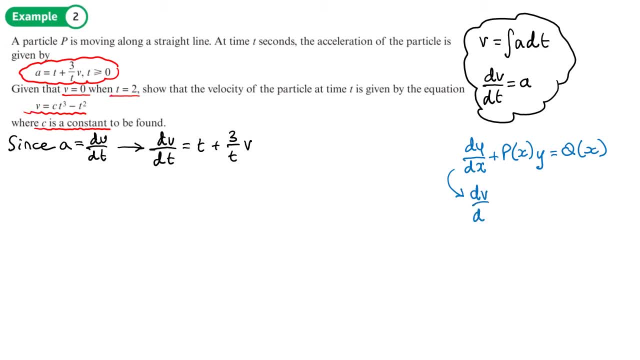 using T, so it'd be dv, dt plus. will it be a function of T? times by V equals a different function of T and it does sort of match up with this. if I rearrange it and solve this, I would use the integrating factor. well, from here, the integrating, 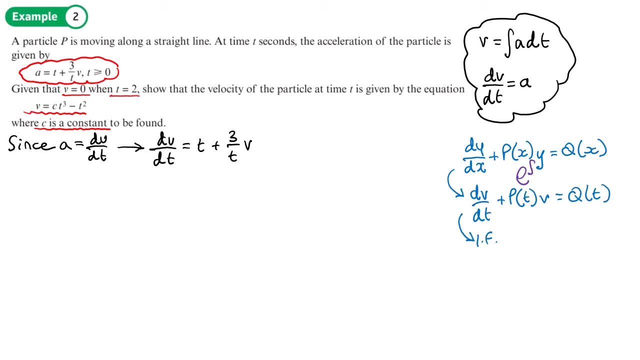 factor would be when you do e to the integral of P, X, DX. so here the integrating factor is going to be P, T, DT. so it's important to get letters to match up. so step number one, let us now, or step number two or three, get it to match up, so we'll rearrange it. 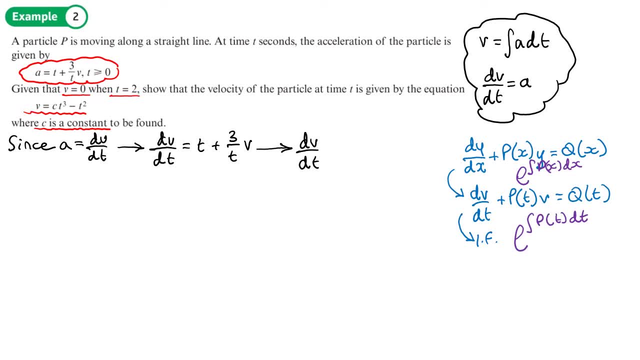 so I'll write dv dt minus 3 over T. V equals T and we're going to solve by using the integrating factor, as we've just spoken about, and the integrating factor is going to be whoops e to the integral of PT. now, PT is this minus 3 T, so it'll be minus 3 T DT. now I can take the minus 3 over as a. 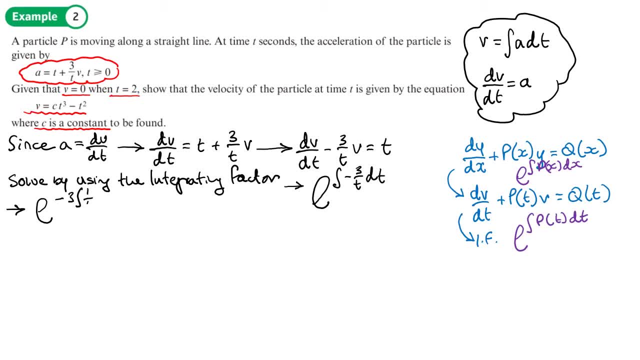 factor. so it just needs me 1 over T DT, which is easy. so now I get e to the minus 3, log T. now if I move the negative 3 over, so it's a power like this, then the e and the log cancel out, just leaving me with T to the power, negative 3. that's my. 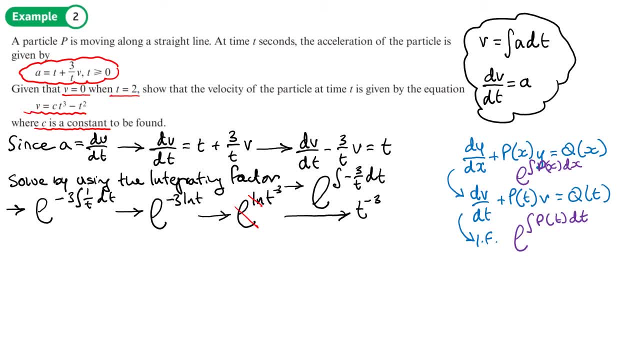 integrating factor. so now I times all the terms in the original equation, differential equation. first of all the differential equation. multiply every term by T to the minus 3, so that will give me T to the minus 3 dv dt, minus T to the minus 3 dv dt, so that will give me T to the minus 3 dv dt. 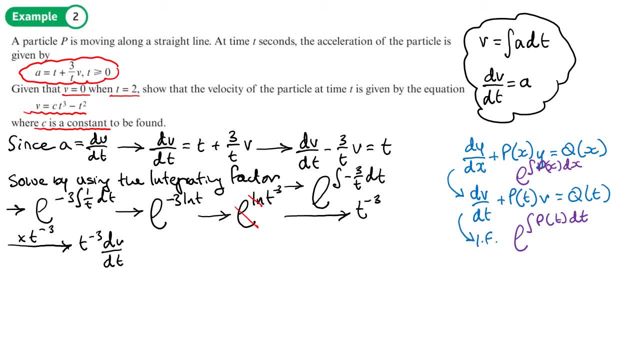 minus T to the minus 3 dv dt times by 3. T or 3 over T. V equals T to the minus 3 times by T. now we need to remember that this is the result of differentiating a product, and that product is going to have this part. so this is where you'd always find U and. 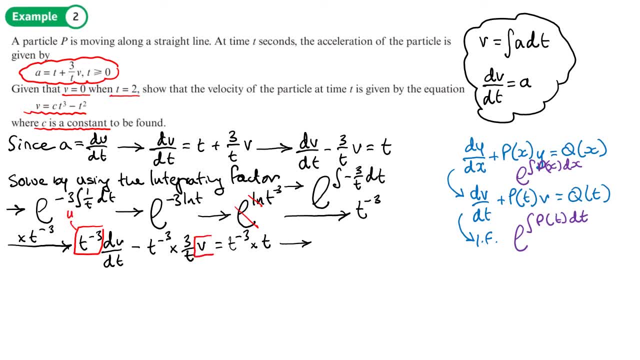 that part of the product, and this is where you're going to find the other part of the product, V here. Now I'll just change the form that it's written in here, just to make that a little bit clearer. So T to the minus 3, dV dt. 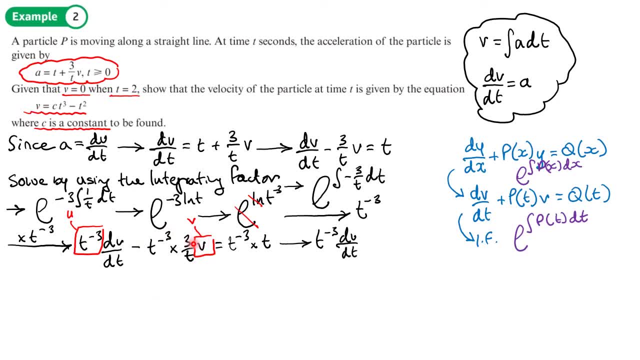 Now, if I look at this part and take that T here, this will actually become T to the power negative 4.. So I'll have negative 3, T to the negative 4, V equals, and then the other side over here will just become T to the power negative 2.. 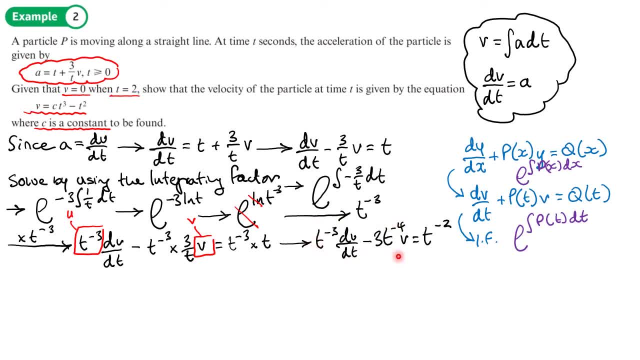 So hopefully you can see more clearly here The result of differentiating a product, because if that's U, this part is what U dash would be, So that differentiating becomes this, and then the V differentiator becomes 1, that's why there's nothing here. 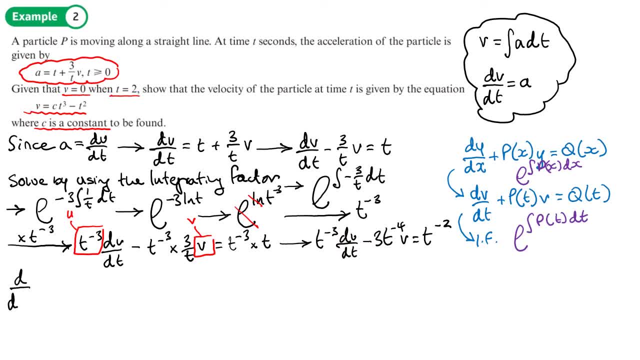 So the left-hand side will write that it's the result of differentiating, with respect to T, this product: T to the minus 3, V, So that's equal to T to the minus 2.. We now integrate both sides. 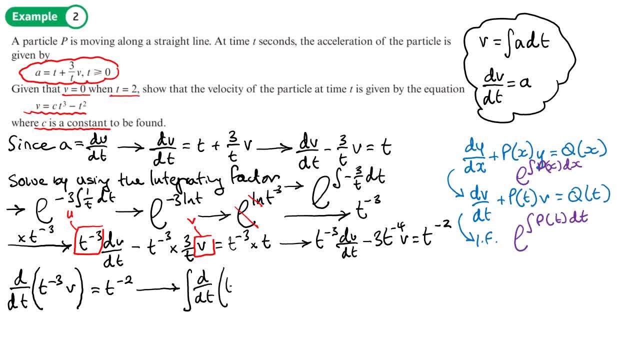 So we will have this. T to the minus 3, V dt equals the integral of T to the minus 2, dt. These cancel out here. So that just leaves T to the minus 3, V equals what we get when we differentiate this. 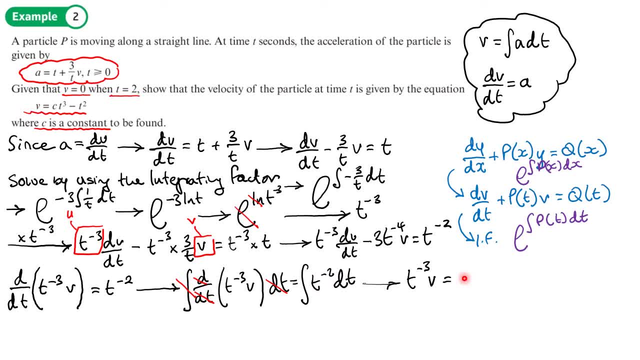 Oh sorry, when we integrate this, So that will become minus T to the minus 1,, plus C, And now we're going to work out what C is, And we can do that using this: when V is 0, T is 2.. 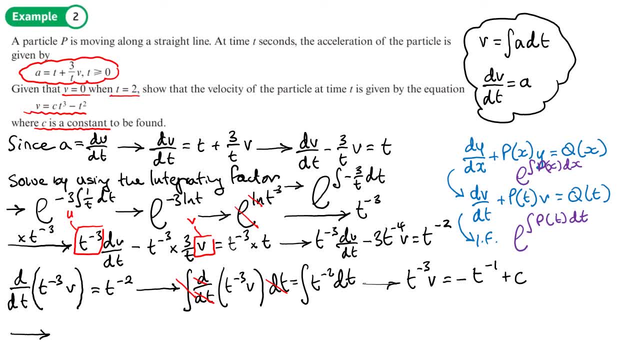 So let's just substitute in: V is 0, and T as 2.. So we will get 2 to the negative. 3, times by 0, equals negative 2 to the minus 1, plus C, So that becomes 0.. 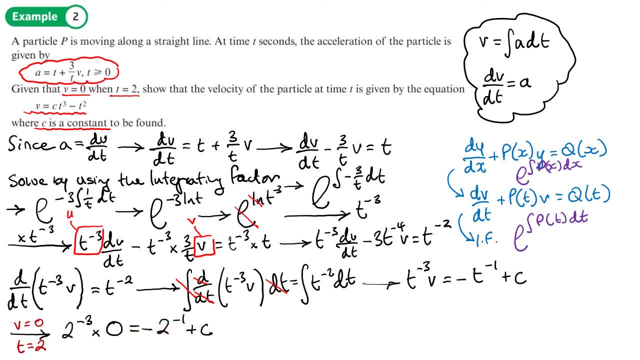 This is minus a half, So that means that C must be equal to a half. So our final answer is going to be that V equals negative T squared plus half T cubed. Now the reason I've ended up with that is because I've basically taken the expression from above here. 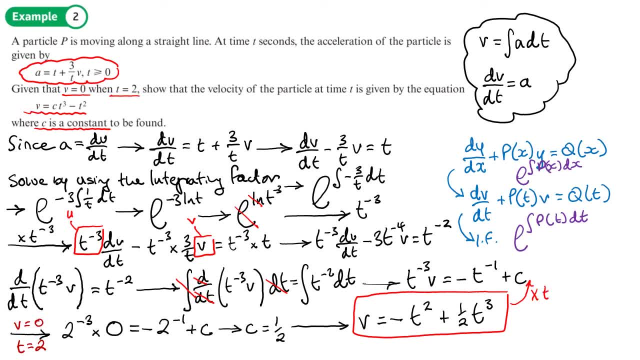 And if you times everything by T cubed, you'll get the expression in the form that they want, because you'll notice there's no negative powers here. So if I times everything by T cubed, that becomes V, This becomes negative T squared. 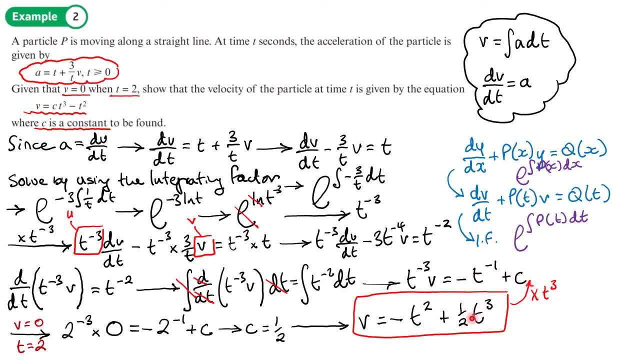 And this will become C times by T cubed, Which is what I've got there. So yet again, we've proved it as required And we've found the value of C. So we might want to probably just say at the bottom here that C is a half. 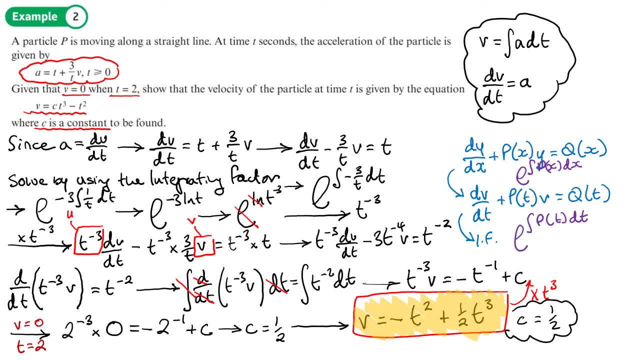 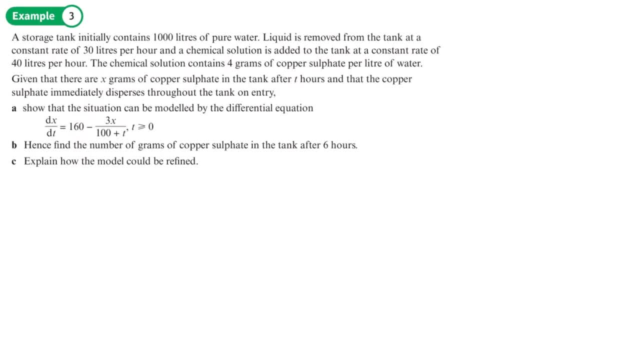 So it's part of our answer as well And just highlight that. Okay, so we've got a storage tank here Initially contains 1,000 litres of pure water. Liquid is removed from the tank. So it's removed at a constant rate of 30 litres per hour. 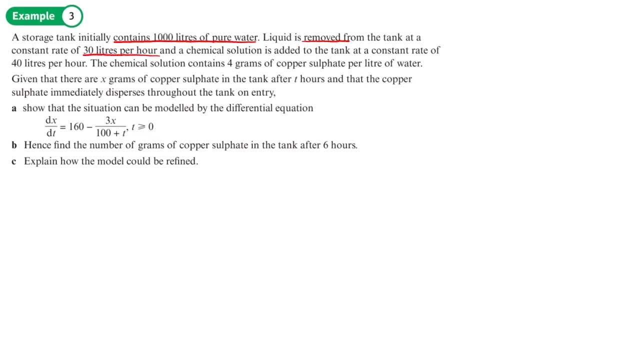 And the chemical solution is added to the tank at a constant rate. So added at a constant rate of 40 litres per hour. The chemical solution contains 4 grams of copper sulphur And the chemical solution contains 4 grams of copper sulphate per litre of water. 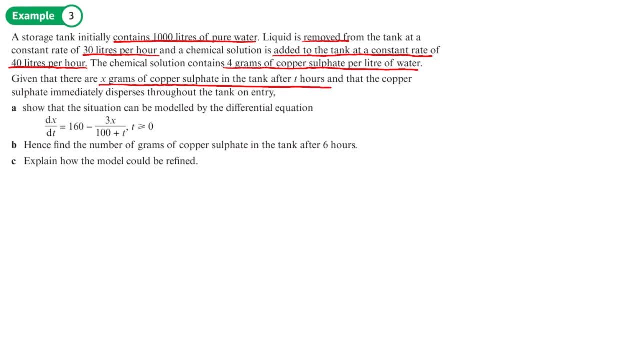 Given that there are x grams of copper sulphate in the tank after T hours And that the copper sulphate immediately disperses throughout the tank on entry, Show that this situation can be modelled by the differential equation that we're given here Right. so first things, 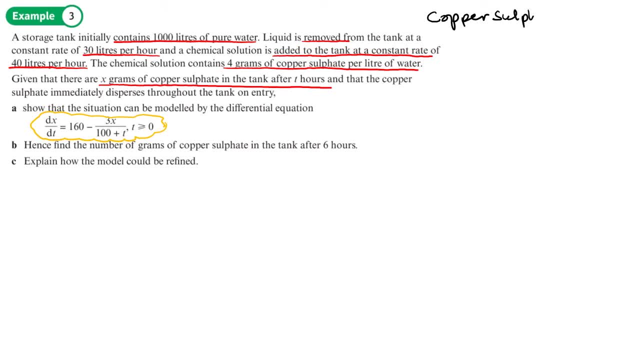 Chemical symbol for copper sulphate, Although not really needed for the question, But it will just shorten some of the writing I need to do: C U S O 4.. So a quick Google allowed me to find that Because I couldn't remember from my A-level chemistry many years ago what it was. 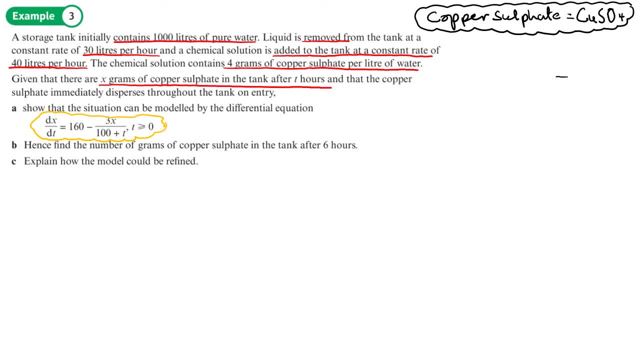 And also a little drawing of what's going on. So I've got some sort of tank here That's got chemicals in it- Chemical, symbol Chemical- being poured into it Like this. So it's already got 1000 litres of water in it. 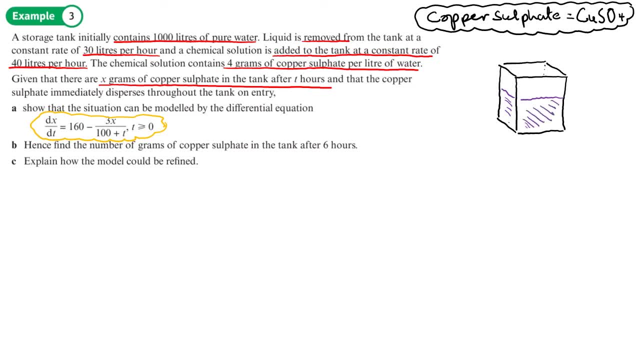 Of pure water. Yeah, So there's 1000 litres of pure water As opposed to impure water. Then we've got liquid being poured in. So let's do like a little cup here And yeah, liquid is being poured into the tank. 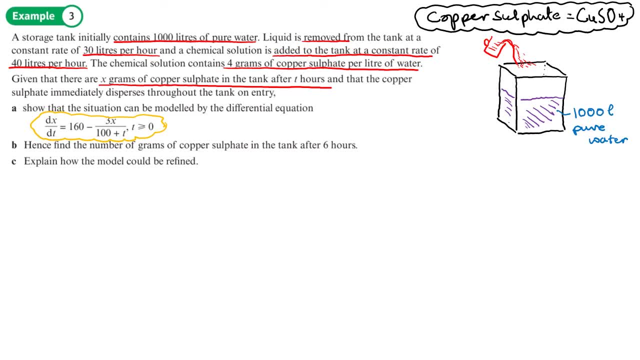 And it's being added to the tank at a constant rate of 40 litres per hour. So 40 litres per hour, But water is also removed from the tank, So let's say there's a little tap on the side here. 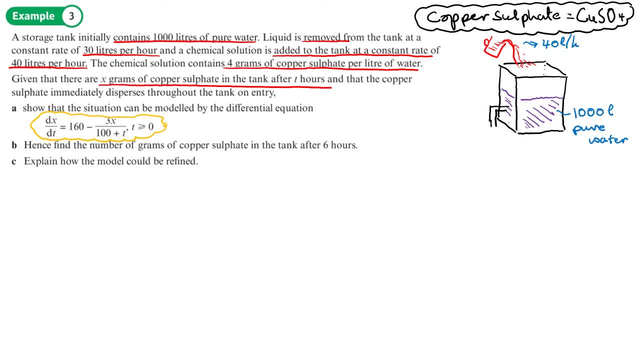 And water is sort of removed from the tank. So let's do some like drips There going down And it's being removed at a rate of 30 litres per hour. So 30 litres per hour And the water that's being poured in has 4 grams per litre. 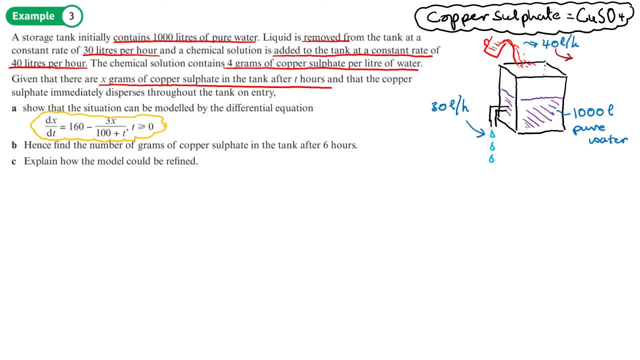 4 grams per litre of copper sulphate, So 4 grams per litre of CuSO4. Our copper sulphate. Okay, So you know the diagram's not really necessary, But helping you know if we've got that. that just helps in terms of answering the question. 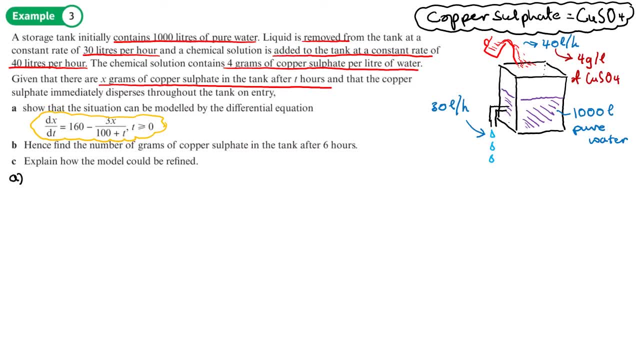 If we can visualise what's going on, Right? So the first thing I want to do Is to work out the amount of liquid in the tank. Amount of liquid in the tank after T hours. Now what have we got? 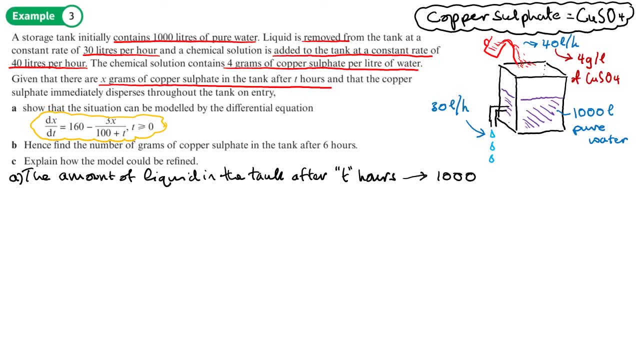 Well, we've got 1000 litres already there And the amount of liquid that's going to be in litres. Then we've got 40 litres per hour going in And 30 litres per hour taken out. So overall we're going to have 1000 plus 10T litres in the tank after T hours. 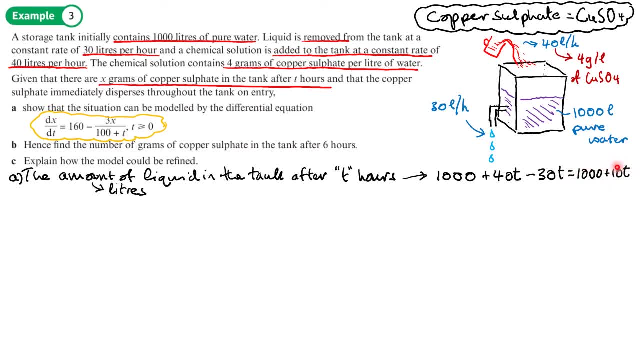 So you can see that every hour what's going to happen. You're going to get an increase of 10 litres, So we'll start with 1000 litres. After an hour there'll be 1010.. Two hours: 1020.. 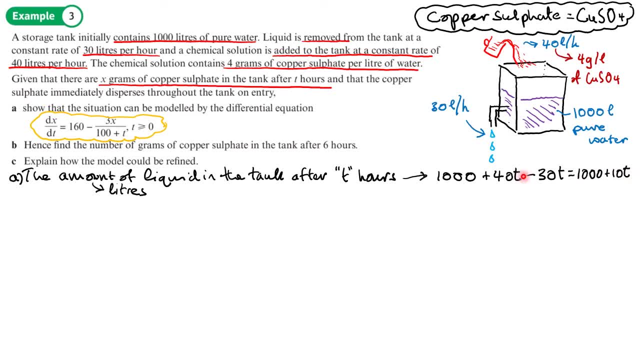 And so on. Now, as the amount of liquid in the container changes, The concentration of the copper sulphate will change. Now it's not going to be the same. It's not going to be like a simple linear thing Because copper sulphate is being added. 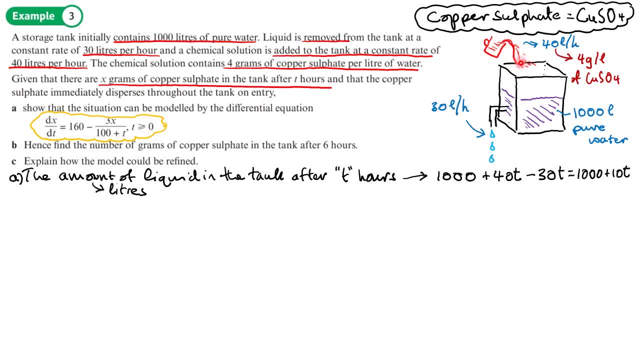 So you're having copper sulphate being added. Some copper sulphate is going to be lost as it's taken out, So it may be that the concentration increases or decreases, And this is what this differential equation is. It's about the concentration. 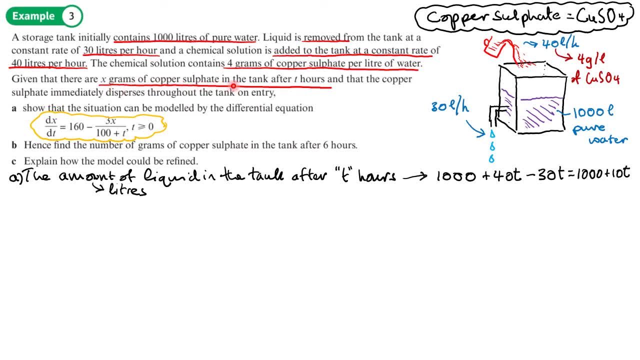 Yeah, which is X. X is like the concentration Of copper sulphate, Of copper sulphate over time. So what we need to do is to work out: Well, what is the concentration of copper sulphate in the tank? Well, that's going to be equal to the amount of copper sulphate in the tank. 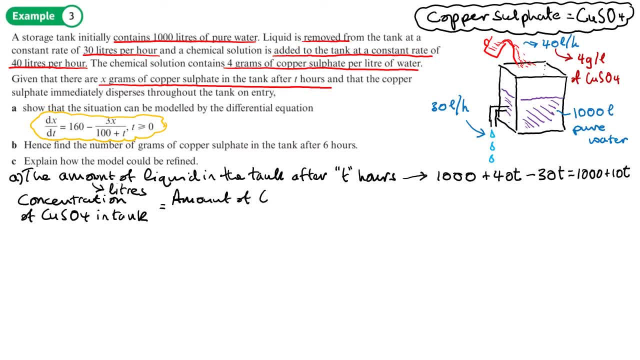 Amount of copper sulphate in tank Divided by the amount of liquid in the tank. Amount of liquid in tank. So the amount of copper sulphate in the tank is given by X, The amount of liquid in the tank is given by 1000 plus 10 T. 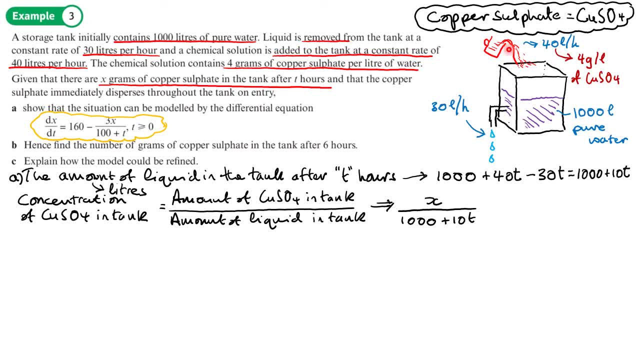 Now that concentration, That concentration will change as copper sulphate goes in And some copper sulphate comes out with this 30 liters that comes out every hour. So if we look at the copper sulphate that goes into the tank every hour, 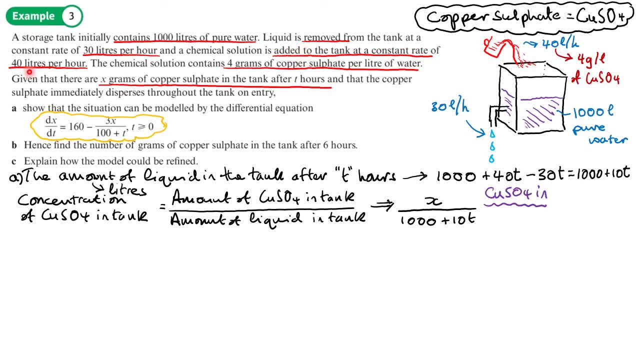 So there's 4 grams in 40 liters, Or sorry, 4 grams per liter. So the amount of copper sulphate that goes in per hour is going to be 4 times 40. So 160 grams of copper sulphate in per hour. 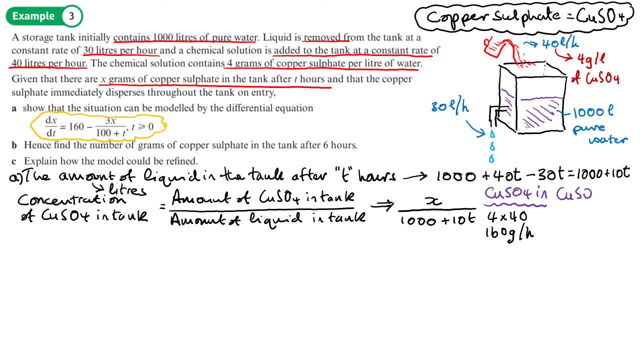 How about the copper sulphate that's coming out? Well, that will be whatever. the current concentration of copper sulphate is Per liter times by 30. Because there's 30 liters coming out per hour, So we need to times this by 30.. 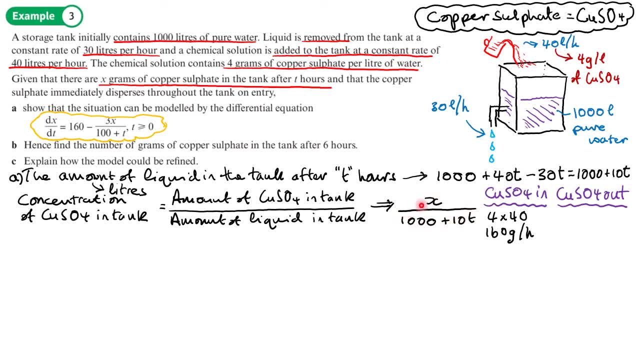 So that's the concentration of copper sulphate in grams per liter And we've got 30 liters, So we need to times it by 30. So we're going to have 30 times by X over 100 or 1000 plus 10 T. 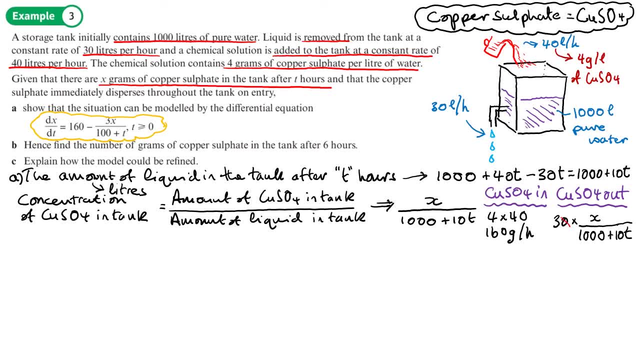 So cancelling down That will give 3X over 100 plus T grams per hour. So the change in the copper sulphate in the tank over time Is the amount of copper sulphate, The amount of copper sulphate that goes in in grams per hour. 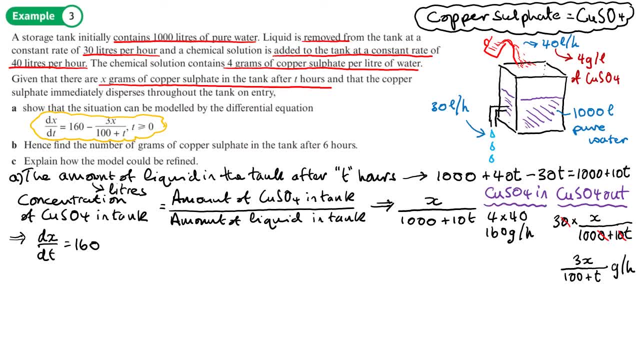 Which is 160.. Take away the copper sulphate that comes out per hour, Which is 3X over 100 plus T. So that's our differential equation proved as required. So now we'll move on to part B. Part B says: 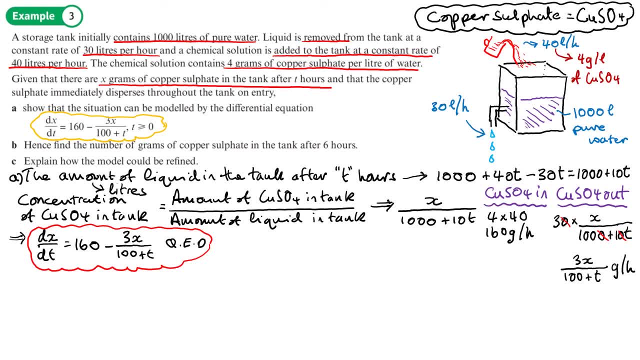 Hence find the number of grams of copper sulphate in the tank after 6 hours, Right? So for part B, The first thing we're going to do is to rewrite this in the form that allows us to use the integrating factor to solve. 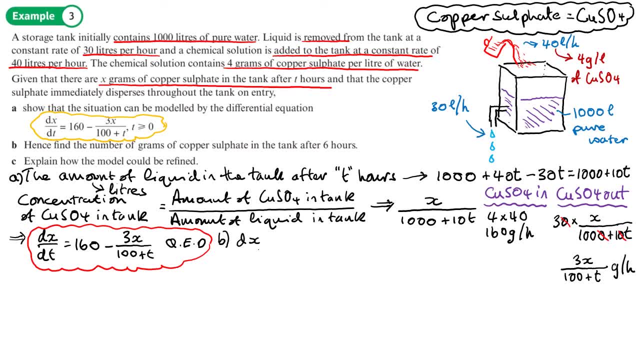 So that will be DX DT. Then we bring over this term. We're going to write it as something times by X, So that will be plus 3 over 100. plus TX equals 160.. So the integrating factor is going to be E. to the power of this. 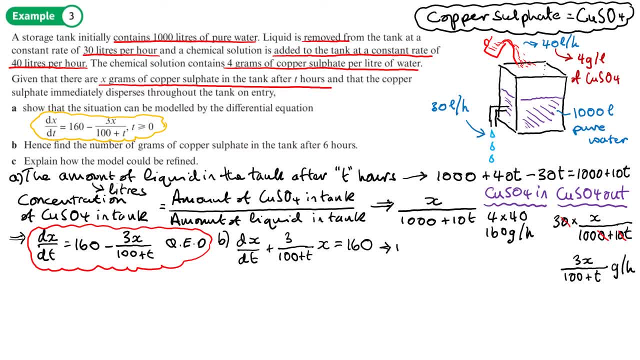 So I'll just write down IF for integrating factor. So that will be E to the power of the integral of. Let's write it: Put the 3 here, 3.. 1 over 100 plus T. DT. Got a bit more space down here. 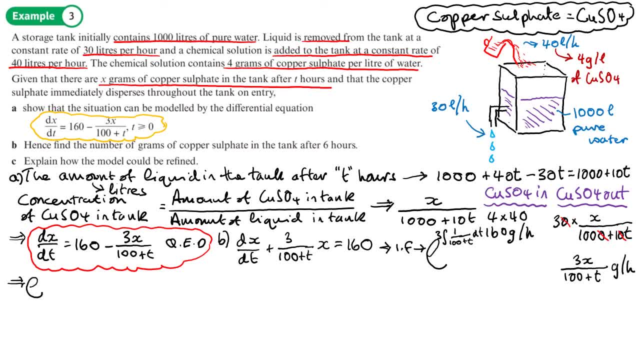 So that will be E to the 3. Then it will be log 100 plus T. Then we can bring the 3 there as a power, Get the E in the log to cancel down And we're just left with 100 plus T cubed as our integrating factor. 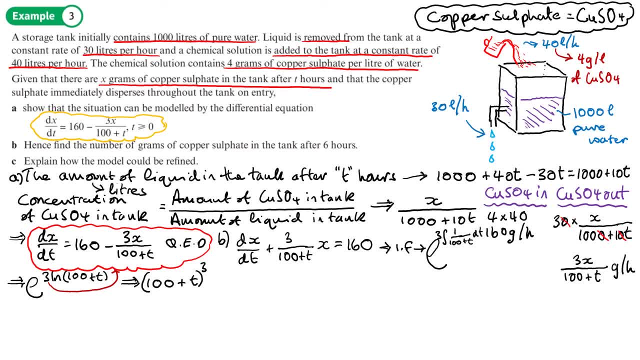 So I'll now take every term of this And multiply it by the integrating factor, So that will give us 100 plus T all cubed DX, DT Plus 100 plus T all cubed times by 3 over. 100 plus TX equals 160.. 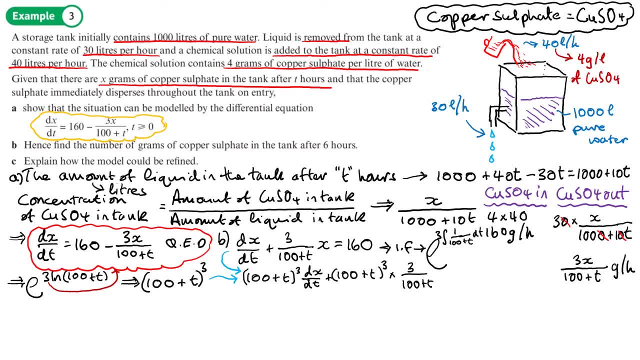 So that will be over 100 plus TX equals 100 plus T, all cubed times by 160.. So I need to identify my U and V. So U is always going to be here beside the DX DT And there's my V. 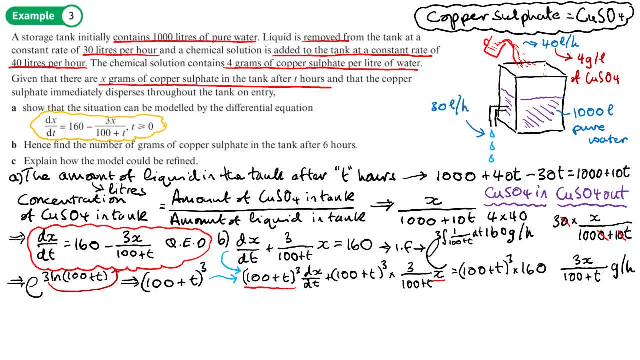 So that left-hand side is what we get when we differentiate with respect to this. We differentiate with respect to this product: 100 plus T- all cubed X, equal to 160.. 100 plus T- all cubed. Next, we integrate both sides with respect to T. 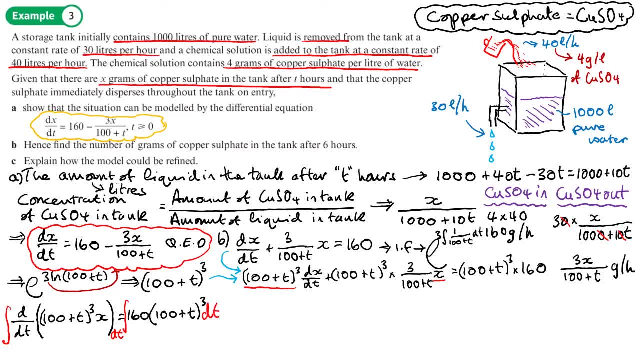 So what will happen is these will cancel out like this. So the left-hand side is now just 100 plus T, all cubed times by X, And then the right-hand side when we integrate it, So we can use the reverse chain rule. 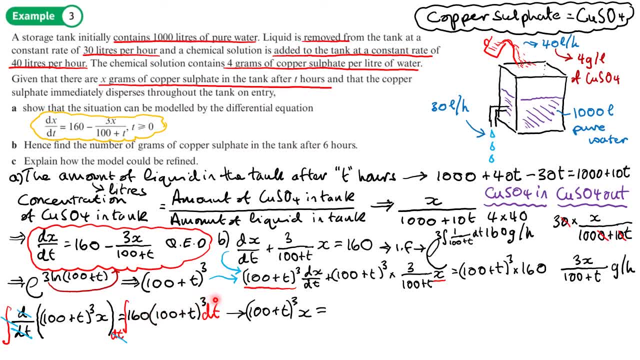 We add 1 to the power, We add 1 to the power, So this will become power 4.. This will become power 4T. Dividing by this differentiator, that's just 1.. So we'll end up with 4T bracket 100 plus T, power 4.. 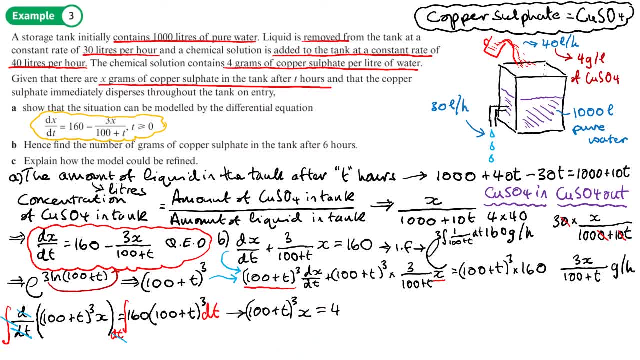 So we'll just write that down: So 4T, 100 plus T power, 4.. Then plus C. Now C is what we now need to work out. Now, to work out C: it says that initially the container contains pure water. 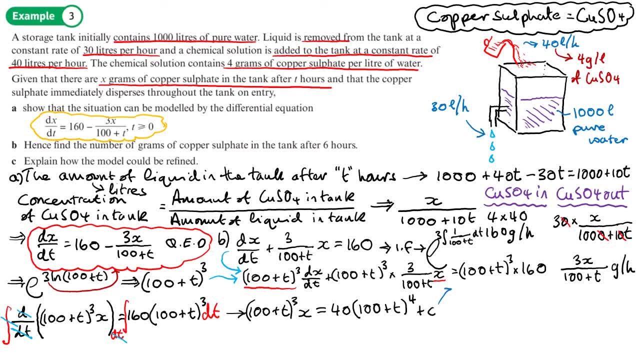 So that basically means that when T is 0, the concentration of copper sulfate is 0.. Okay, So that bit was important about it containing pure water at the start. So we're going to replace this X with 0. 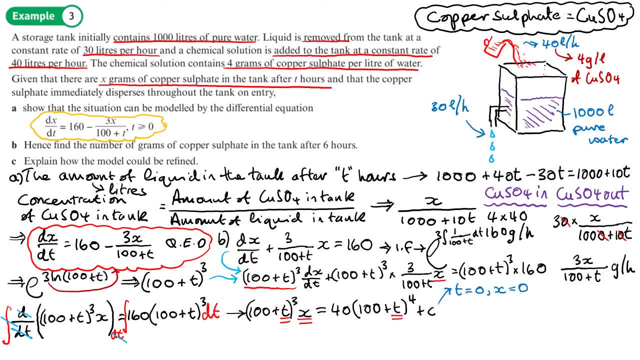 And this T with 0. If we do that, this part here just disappears. That becomes 0. So we have 40 times by 100 to the power 4.. So C will equal negative 40 times by 100 to the power 4.. 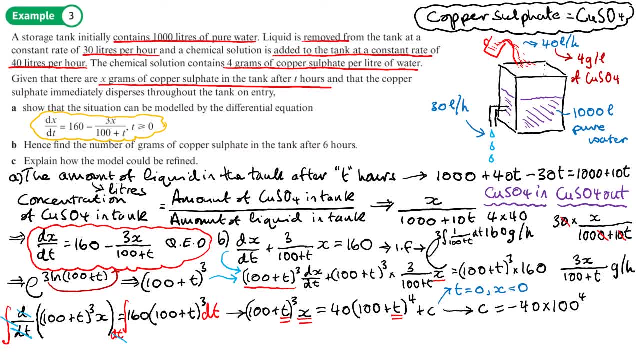 So that's our value of C. So adding our value of C and rearranging, we'll get X equals. So this will be 40 times by 100, plus T, to the power 4.. Adding C, which is minus 40 times by 100, to the power 4.. 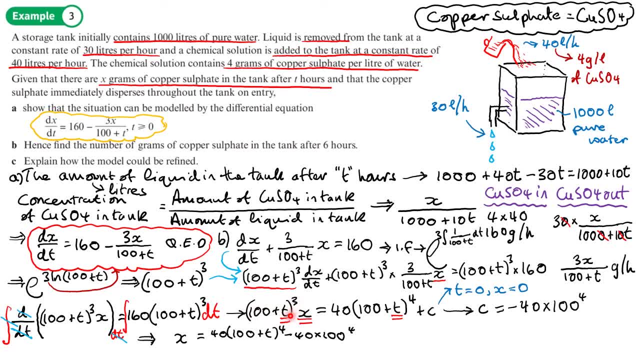 And I'm dividing both sides by 100 plus T cubed, So all over 100 plus T cubed. I want to find the concentration or the amount of grams of copper sulfate when T equals 6.. So I've already done this. 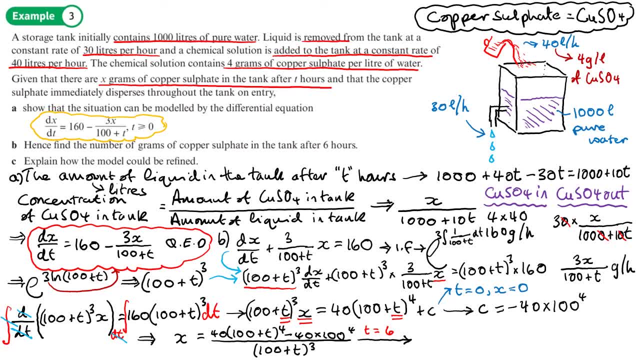 If I put T equals 6 into that equation, I'll give you my exact answer, and then I'll round it to three significant figures. So I'll get 881.5228.. So let's give that as 882 grams. 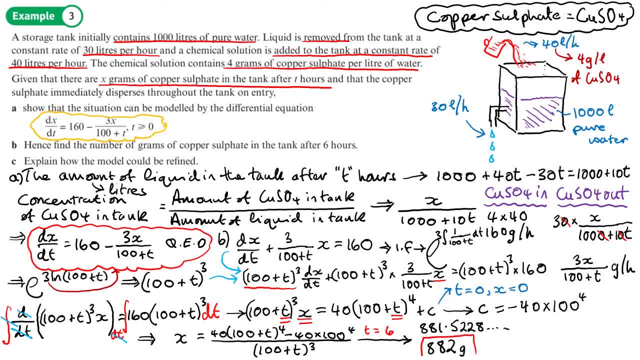 And there's a three significant figure answer. So there's my answer for part B. You can see there's quite a bit we need to do. There's quite a bit we need to do in that in part A and part B. 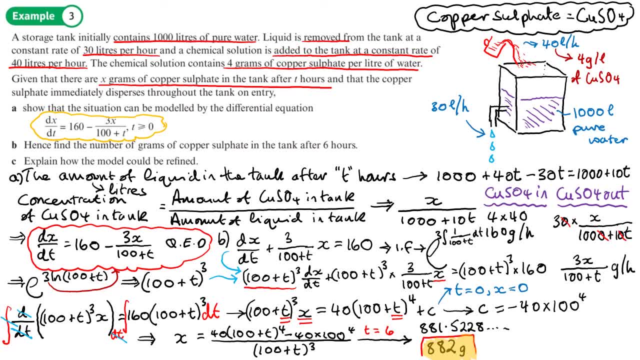 So let's just highlight the fact. that's part B, just in case. And in part C, how could we refine the model? In other words, what could we include or take away from this to make it more realistic? Now, as long as you give any sensible answer that's related to the question, you'll get the mark. 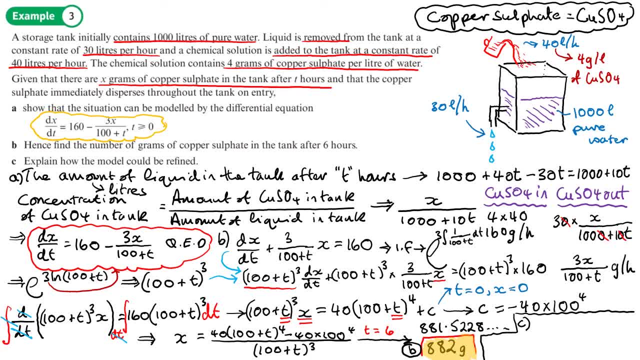 So, for example, it was assumed it says that the liquid or the copper sulfate, it says it immediately disperses into the hole There we go, Immediately disperses throughout the tank on entry. Well, in reality it doesn't immediately disperse. 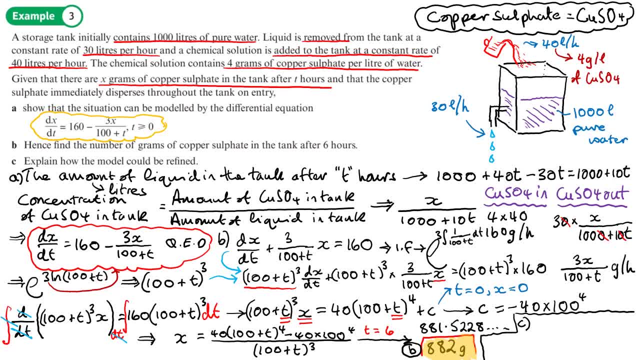 Okay, Some of it may take a while to dissolve, So we might talk about this. immediate dispersion is an issue. Yeah, it's not realistic. So we might want to take into the fact that the copper sulfate doesn't immediately disperse in the tank. 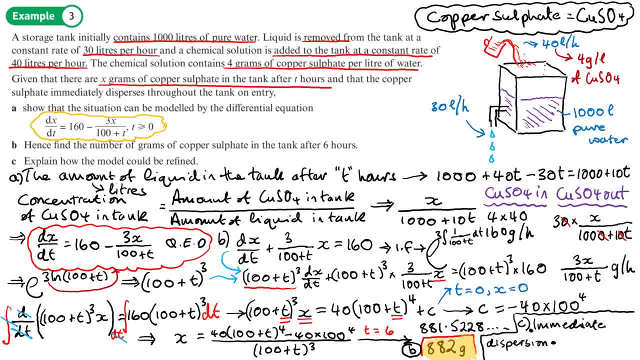 That could make it more realistic. We could talk about the fact that, well, it says that it all dissolves. Does it all dissolve? It may take a time for it to dissolve, So we need to maybe talk about the fact that, you know, the copper sulfate doesn't all dissolve. 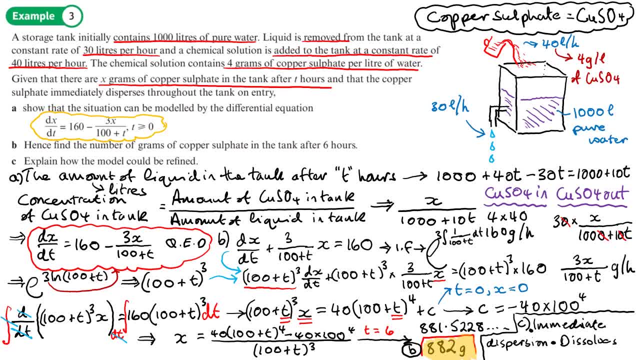 Some of it may sink to the bottom. There may be more concentration in different parts of the tank. So you know, we could talk about that as well. We could also talk about the fact that this model sort of assumes that this tank is going to carry on filling forever because there's going to get more and more liquid in it- 10 liters per hour. 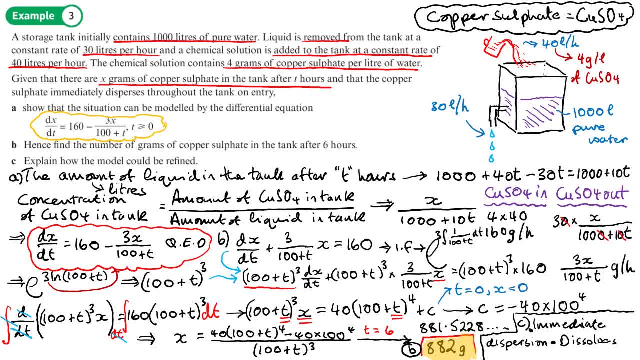 So you know, we could talk about the fact that the amount of liquid that's in the tank, you know we might say, right, this is only valid for a certain amount of time. Yeah, so here are just three examples. 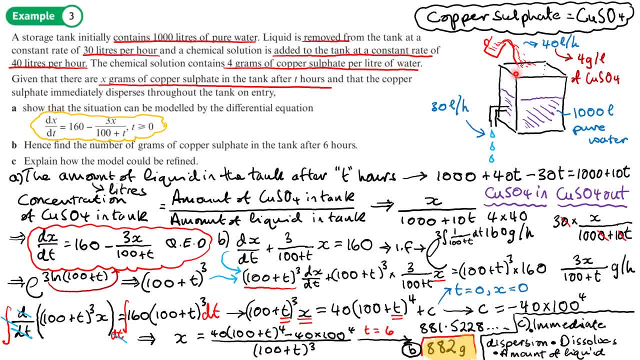 But any example or any reference to the question. so talk about the amount of liquid in the tank, Talk about the concentration of liquid in the tank, Talk about the fact that it's like pure water. You know, is it going to be pure? 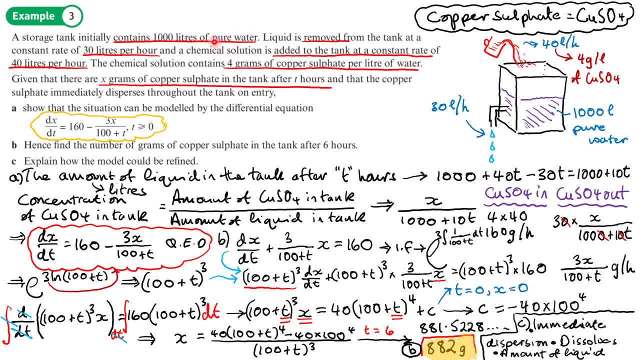 Is there going to be some remnants of copper sulfate from before? Talk about the fact that you know it talks about time. Yeah, Talk about how it's immediately dispersed throughout the liquid on entry. Any of these things will get you a mark. 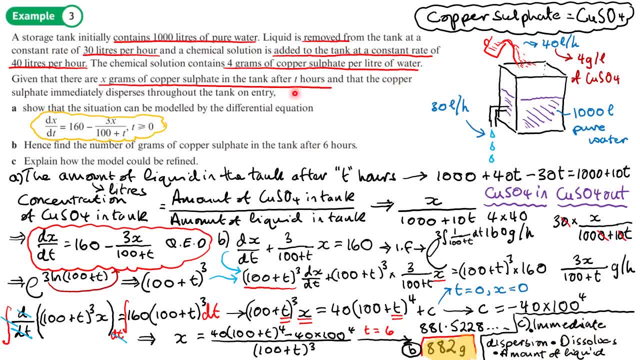 It's always worth reading through the question again and see what things are mentioned to simplify the question. Yeah, those are the types of things that you want to mention here in this part C- Any simplifications here. You should now be able to do exercise 8A.